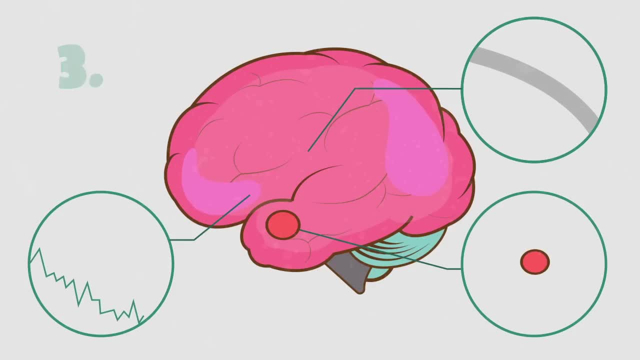 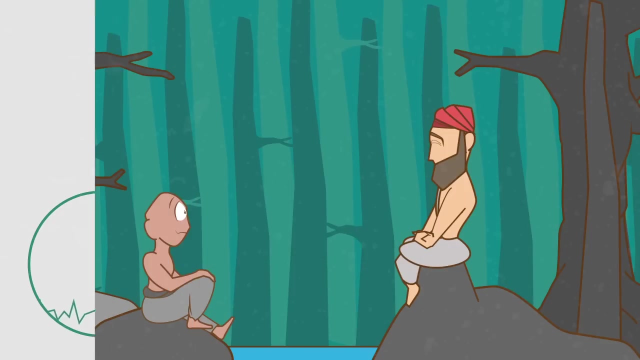 which in turn enhanced sense perception. These were startling discoveries, and it became clear that there was something to this ancient practice after all. But it's not just neuroscience. The field of psychology also owes some recent developments to this eastern philosophy. The mystics of old times claimed this simple fact. With regular insight, you'll see that your 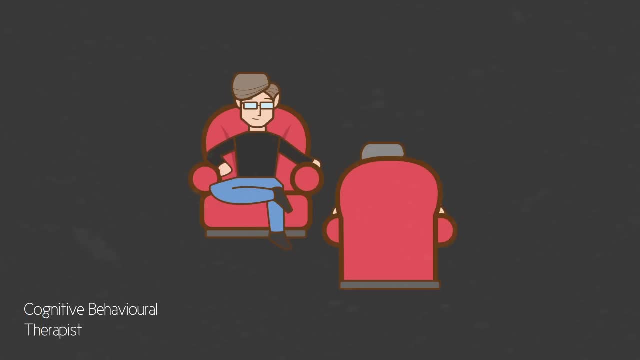 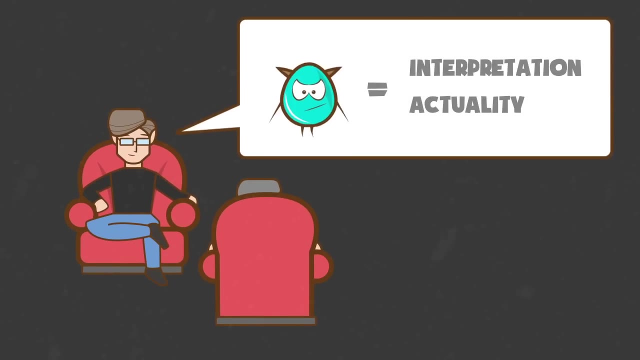 thoughts are not real, And the recent success of cognitive talk therapy uses this exact same strategy. The subject learns to see the falseness of their own repetitive thinking. They are simply an interpretation of what is going on, not the actuality of what's going on. 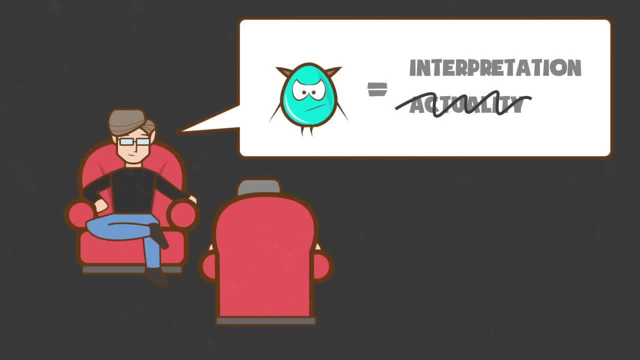 What's the difference? you might ask. Well say, someone next to you makes a sarcastic remark. This may trigger you to start thinking about a number of possible explanations, and they could all be completely false. For example, she did that on purpose. 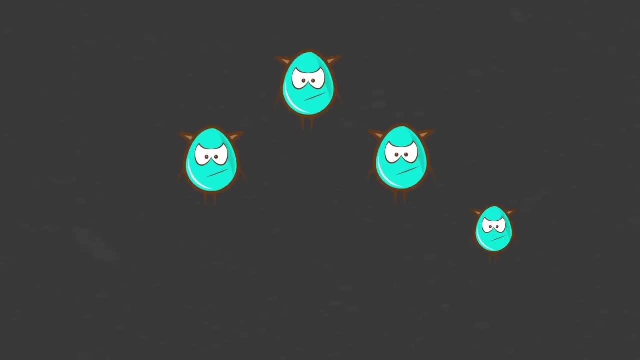 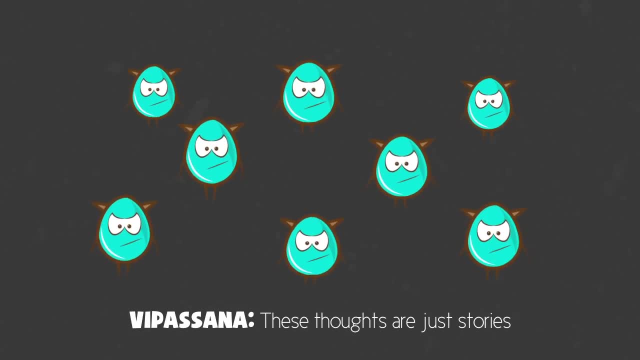 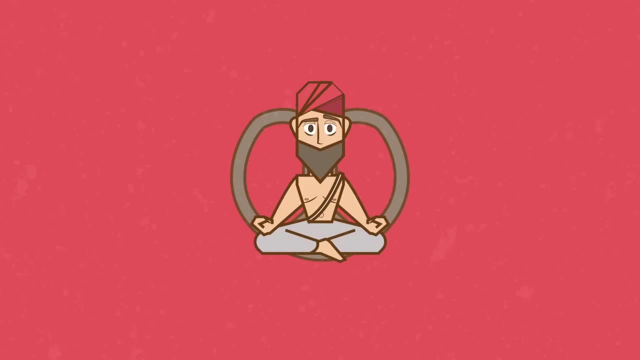 they stop multiplying so quickly. But don't be disheartened, It takes practice. By the way, you don't necessarily have to look like a yogi or sit like a pretzel to meditate, So whether it's breathing meditation, watching meditation, dancing or fishing meditation, 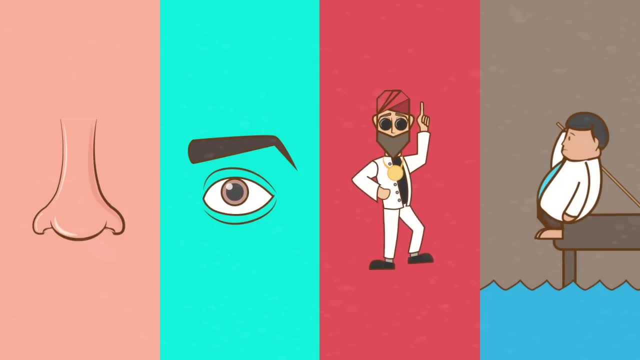 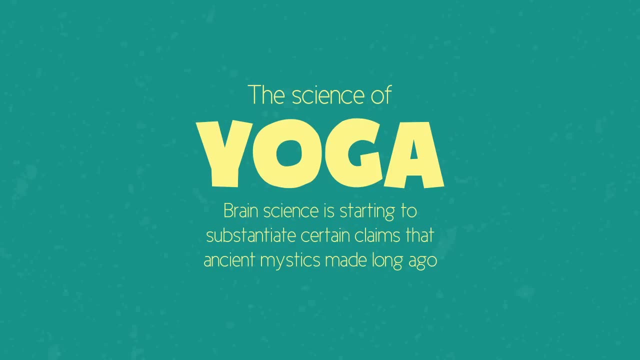 whatever clears your mind is a great place to start. All of these techniques contribute to a healthier mind. There is something that brain science is starting to substantiate, and it's what ancient mystics said all those years ago.